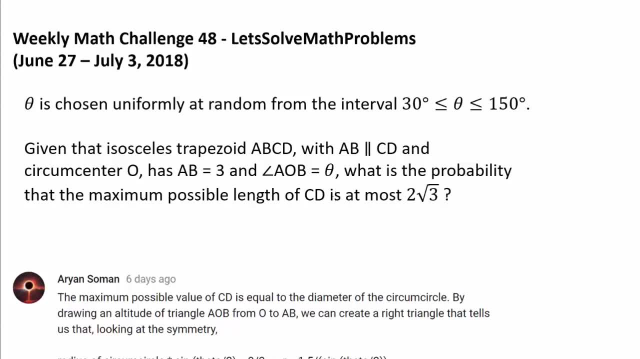 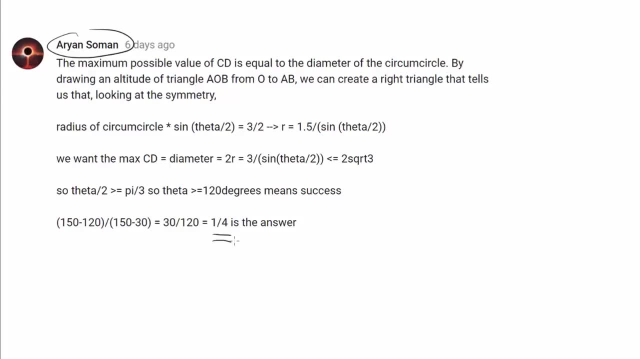 length of CD is at most 2 times the square root of 3.. Before I go on, I want to recognize Arlyan Soman for being the very first person to correctly answer last week's challenge. A huge shout out to Arlyan Soman, Let's try to arrive. 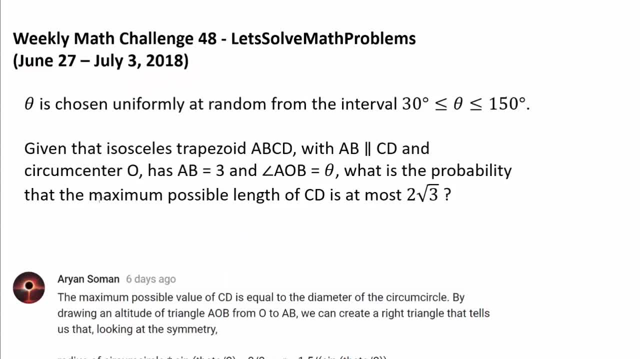 at the same answer of ¼, And this is worded in a strange way. Maximum possible length of CD is, at most, 2 times square root of 3.. What is this talking about? So let's start by dissecting this statement a bit, to make sure we understand what we want to do. 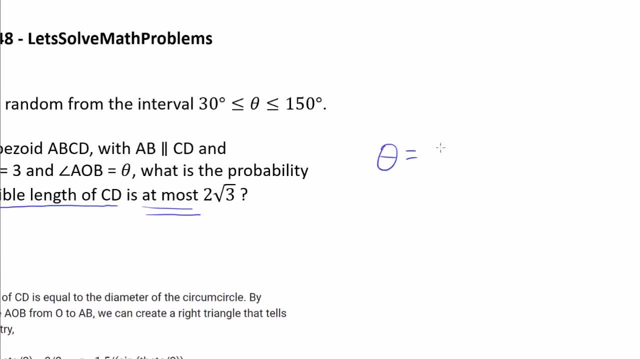 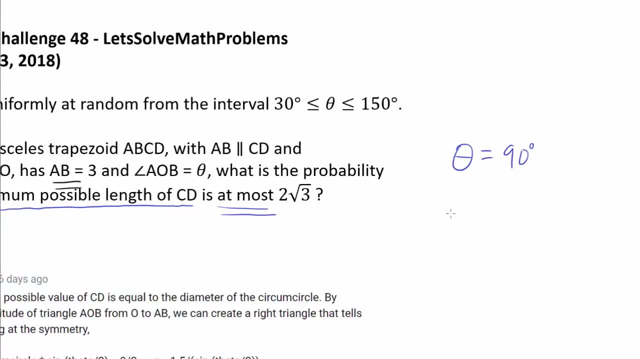 So, For example, let's say data is 90 degrees. We know data is between 30 and 150, so 90 should work. So in this case we have AB of 3, so let's draw AB. so we know this thing. 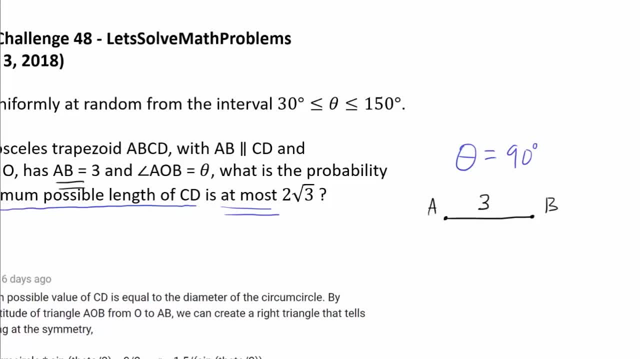 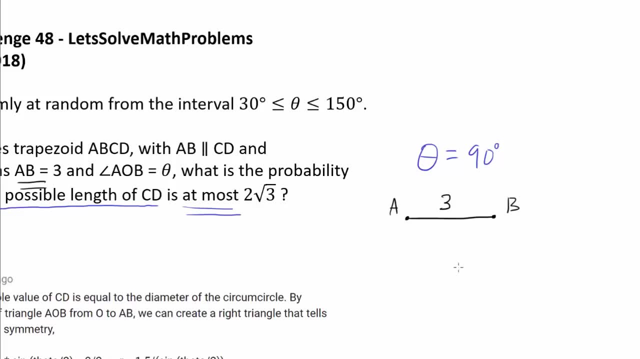 has length of 3. And we know we have the circumcenter O and AOB is data, in this case 90 degrees. So let's put some circumcenter O and we know this is 90 degrees, AOB is: 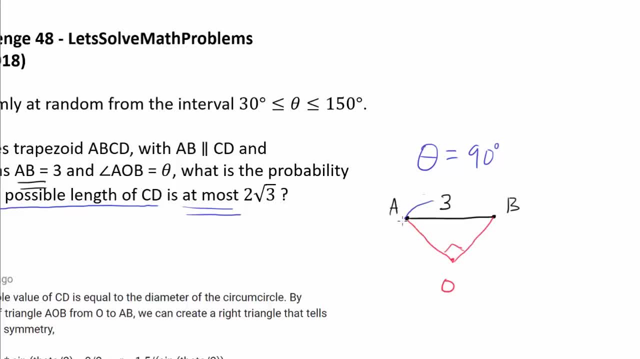 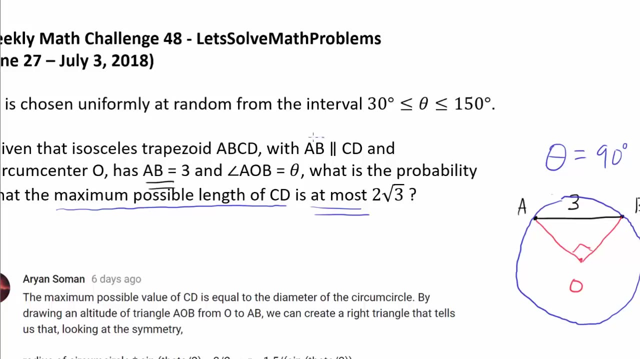 90. So we have this and we know we have a circumcircle that goes through A and B with the center O. So we have a circle that looks like this And we're looking for the maximum possible length of CD And, of course, ABCD is isosceles, trapezoid and AB is parallel to CD And one. 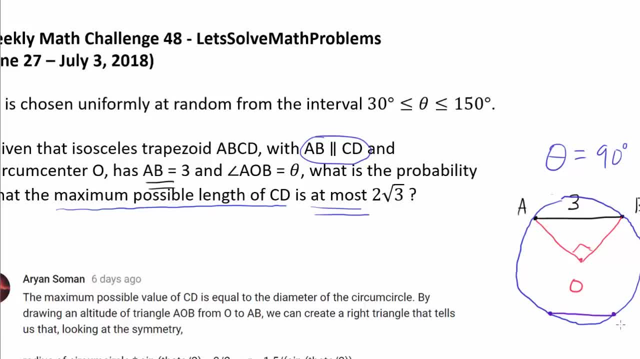 possible way of drawing CD is like this. So this is one possibility for CD and you see this isosceles trapezoid: A, B, C, D. So that's one possible way. Or we may have C D. that looks something like this: 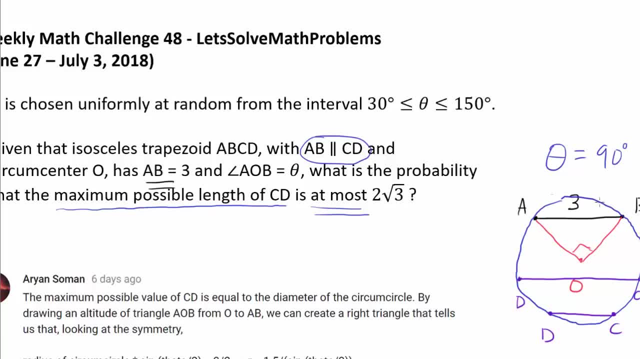 This may be another way of drawing C D, And this may be another way of drawing C D, But we're looking for the maximum possible length of C D. So what is the maximum possible length of C D in this case? 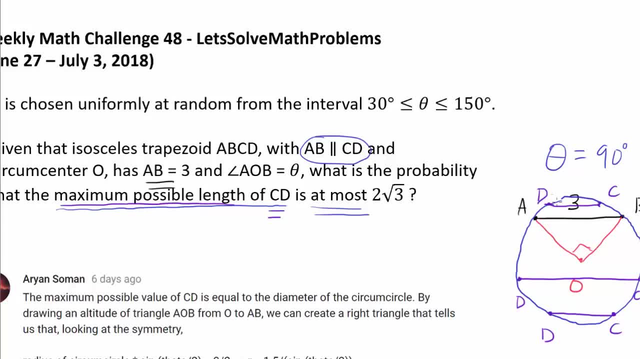 Well, every C D is a chord of a circle, So every C D is a chord of the circumcircle. So we're looking for the maximum possible length of the chord And of course that's going to occur when C D is the diameter. 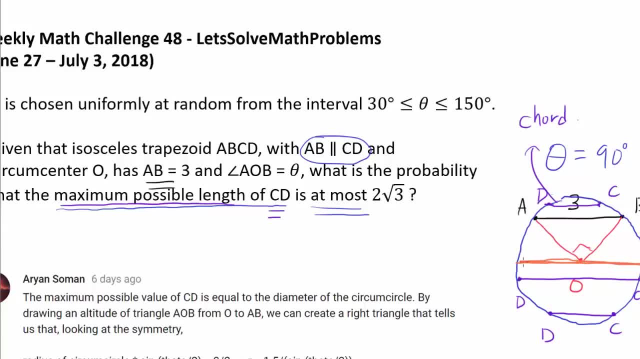 So when we have C D as the diameter of circle O, we are going to have a maximum possible length. So basically, the statement maximum possible length of C D and the diameter of circle O are the same thing. We are talking about the same thing. 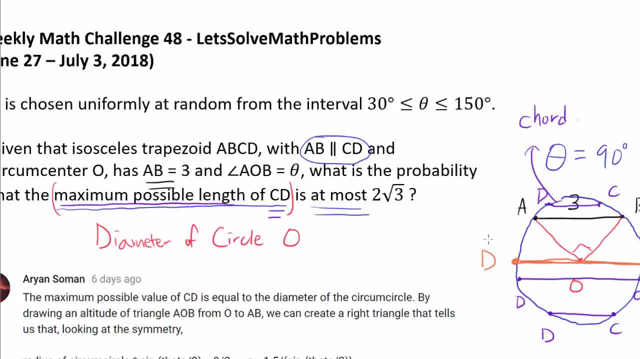 So we are trying to find the probability that the diameter of the circumcircle is N-most two times square root, So three or less than or equal to two times the square root of three. This is much easier to understand than the original statement. 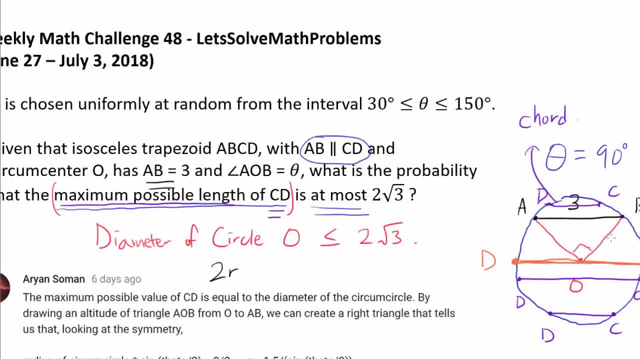 And also because diameter of circle is two times the radius. If you let the radius be R, you know that's less than or equal to two times square root of three is same thing as R is less than or equal to square root of three. 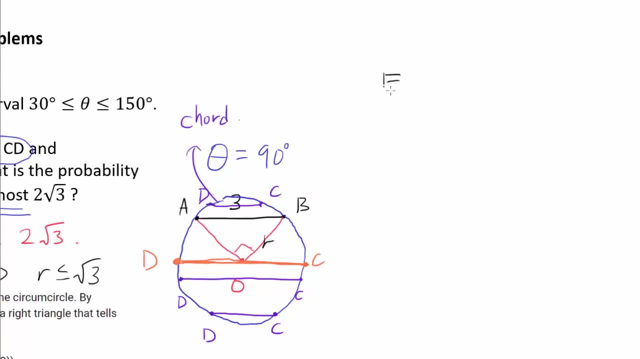 So, basically, we can rewrite the question like this: for what values? So? for what values of data? For what values of data is R less than or equal to square root of three? Once we find this, we can find the probability based on the fact that data is in between 30 and 150.. 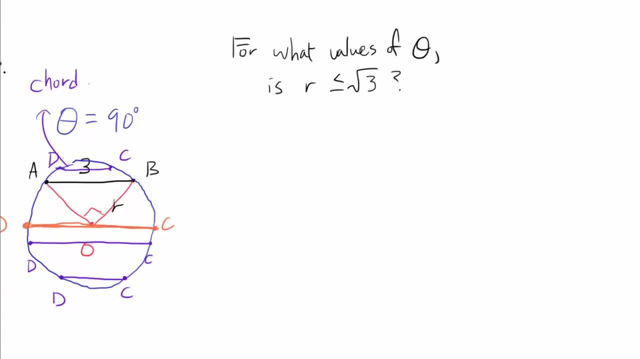 So let's focus on this question. For what values of data is our radius less than or equal to square root of three? So let's try to find some relationship between data and R. One thing we have to keep in mind is that AB is always equal to three. 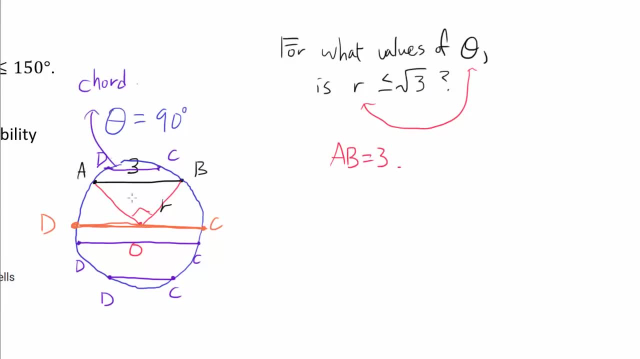 So let's write that down. So AB is always equal to three, So let's write that down. So in this case we have AB of three and data of 90 degrees And let's see what happens if data increases. If data goes up, let's think about what happens to the radius. 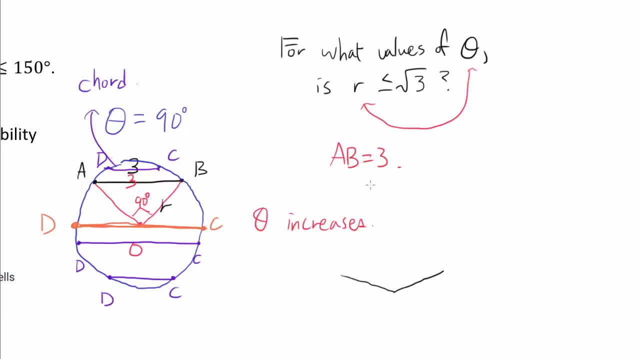 Well, if data increases to become an obtuse angle, then to keep AB length of three, you don't have to go as far out, We don't have to go as far out from the center. So we know this as length of three. 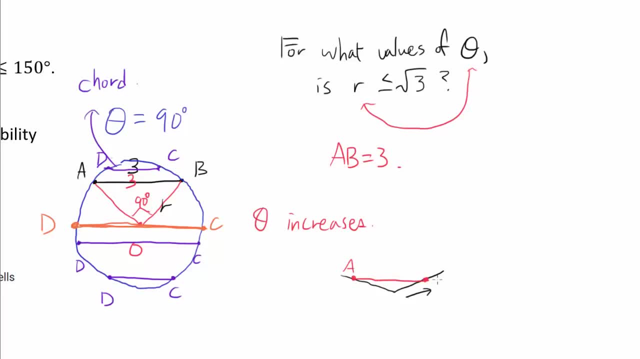 So we know about this- is going to be a length of three, So AB. So we know this is the radius, So our circle is going to be smaller. So our circle is going to look like this: And if data decreases, if data decreases so let's say it becomes acute. 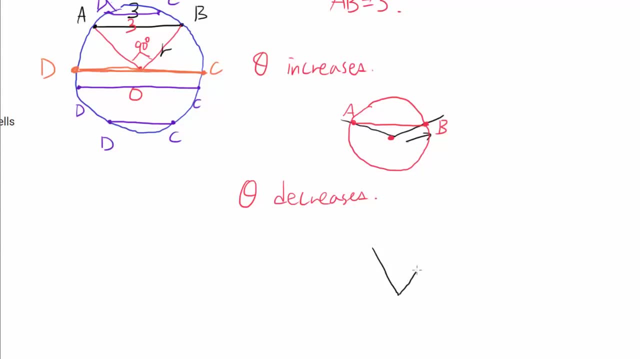 So if we have data looking something like this, then we are going to have to go farther out for AB to measure three. So now we have AB measuring three and our circle looks something like this. So in this case radius went up, So we quickly see that. 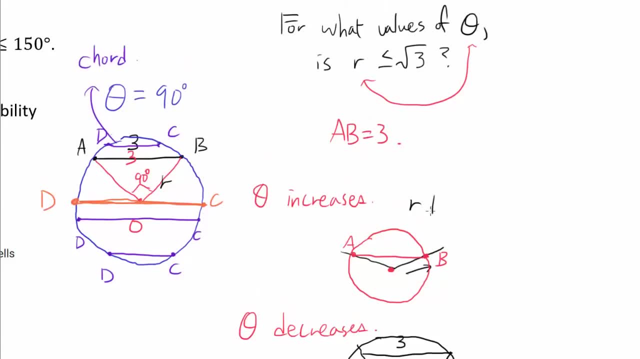 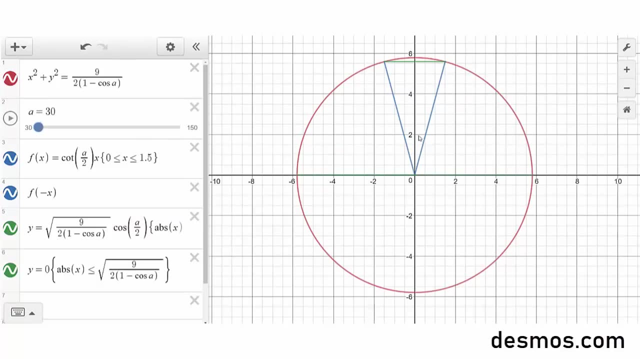 For larger values of data, radius is going to go down And for smaller values of data, radius is going to go up. Just to solidify the visual intuition, I made this graph from Desmoscom And, as you see, this is the value of data. 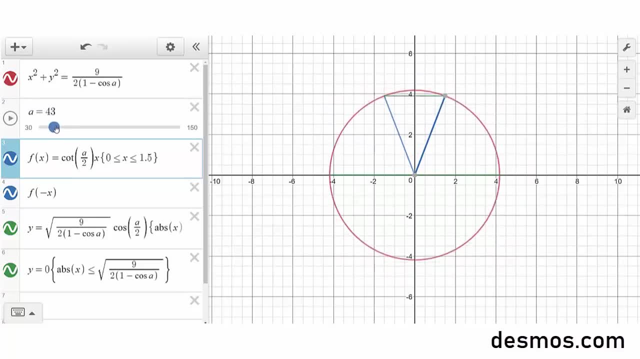 That's the angle between these two lines. And as our data increases, our circle goes down, keeping this distance always three. So from negative one point five to one point five. So this always has length of three. And as data Becomes more and more obtuse, our circle decreases or the radius decreases. 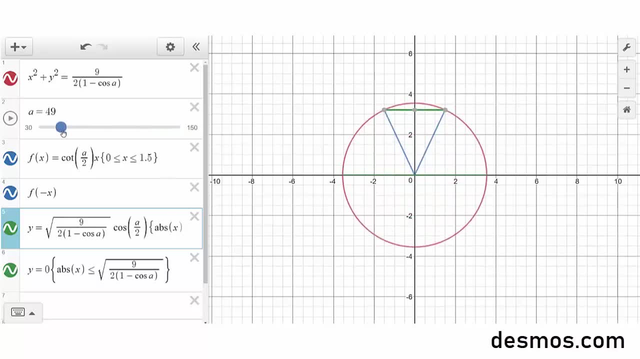 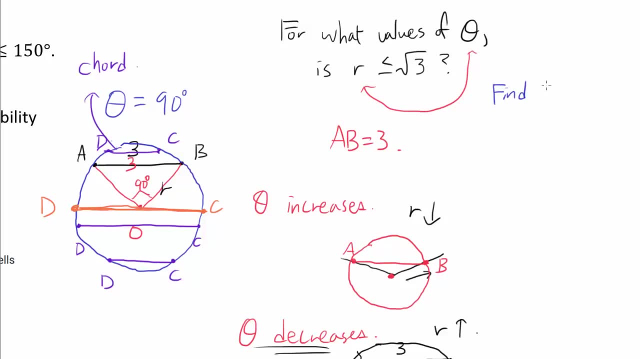 And as our angle gets smaller and smaller, our radius gets larger and larger. So one way of finishing up this problem is like this: If we can find the value of data such that, such that the radius is exactly equal to square root of three, 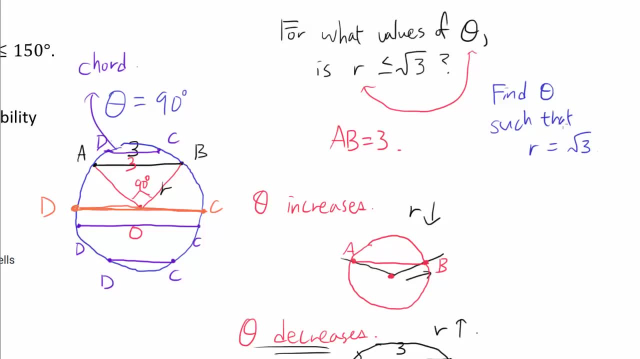 So if we can find the data such that radius is equal to square root of three- So let's call this data some data, not- then we know for data greater than or equal to data, Not r- is going to be less than or equal to square root of three, because as data increases from this data, not our radius is going to go down. 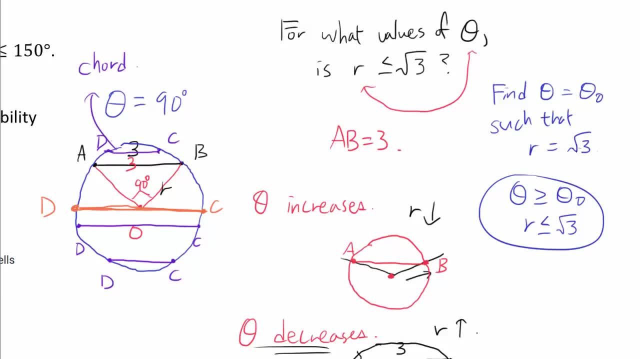 So once we find the data such that r is equal to square root of three, we are done. We know exactly what we're talking about in terms of what kind of values of data satisfy our requirement. So let's finish this up. So we have a b length of three. 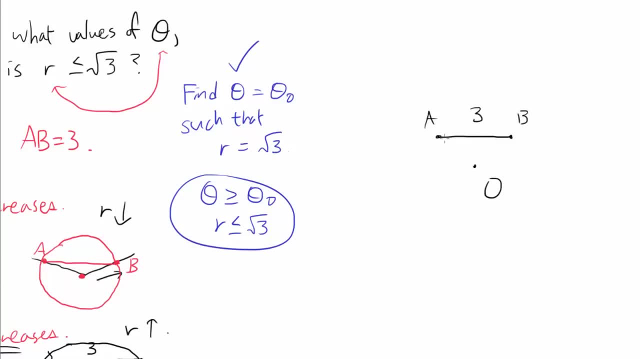 So a, b has length of three. We have some center all And we have the radius Measuring exactly square root of three. So this is also measuring square root of three And we want to find this data And, of course, law of cosine looks like the way to go. 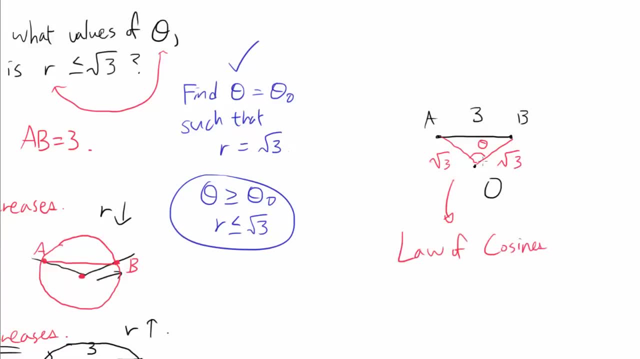 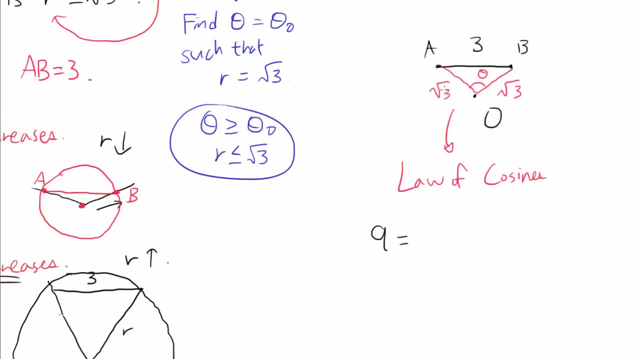 Law of cosines, because we know all three sides and we have one missing angle. So let's just apply law of cosines. So we know ab squared or nine is equal to square root of three squared plus square root of three squared minus two times square root of three times square root of three.